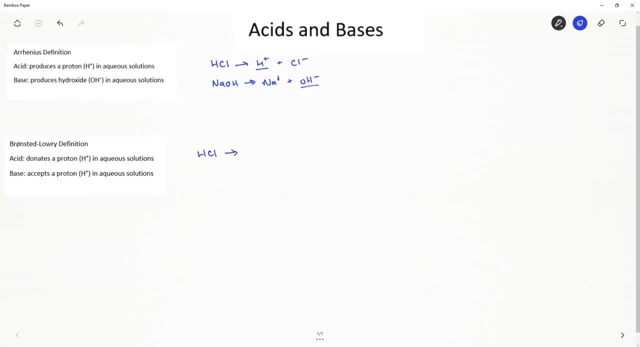 Our hydrochloric acid in aqueous solution still is an acid under our Bronsted-Lowry definition. It's still donating a proton For our base. let's take a look at ammonia, because it does not fit our Arrhenius definition. 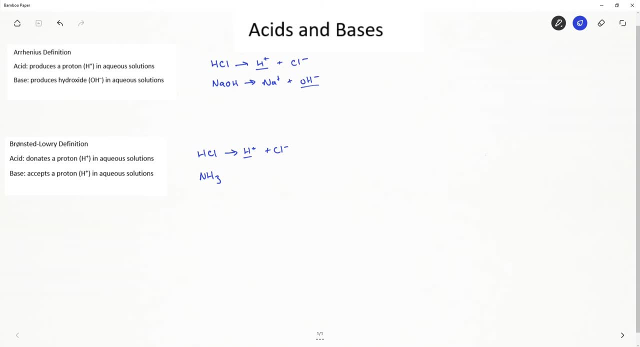 However, it will fit our Bronsted-Lowry definition. So for Bronsted-Lowry, base ammonia must accept a proton and it does this by accepting a proton from water. It forms the acid. It forms the acid, It forms the ammonium cation and what's left is hydroxide from this OH left in water. 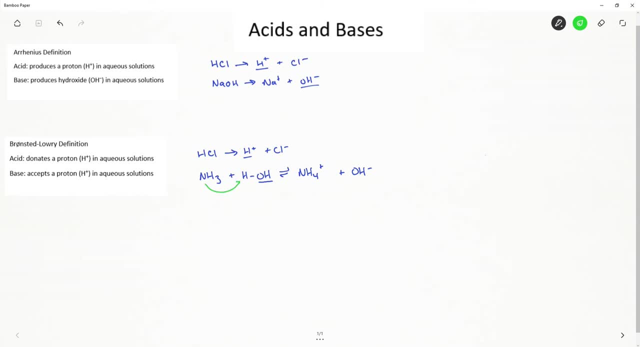 So our ammonia molecule has accepted a proton from water to become ammonium. There is one more definition that I want to go over, and that is the Lewis definition for acids and bases. And yes, this is the same Gilbert Lewis of Lewis structure fame. 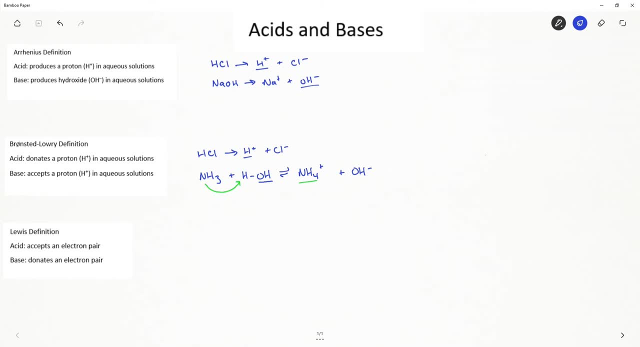 Now for the Lewis definition. an acid is going to accept an electron pair and a base is going to donate an electron pair. Let's take a look at the reaction of aluminum trichloride with a chloride anion. We will start by drawing our Lewis structures. 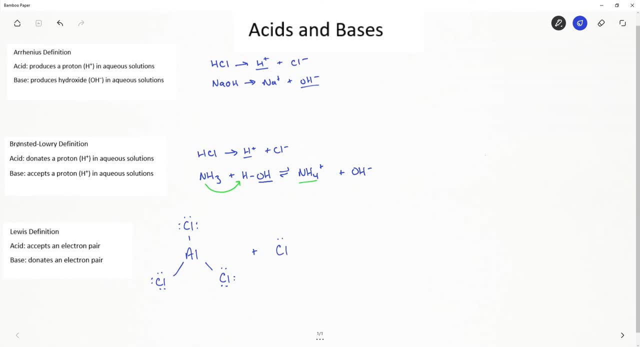 You will notice in these Lewis structures that aluminum does not have a complete octet. It will accept an electron pair from chloride. Chloride donates that electron pair. Therefore the aluminum trichloride acts as the acid and the chloride anion acts as the acid. 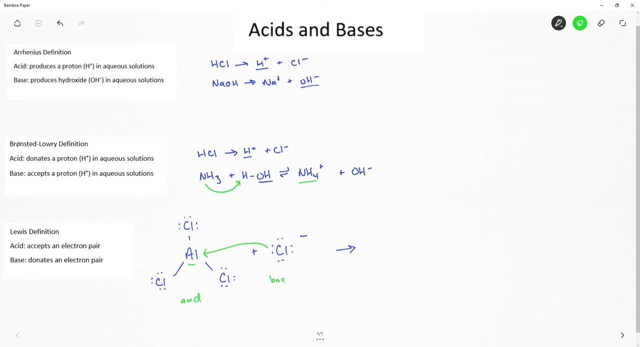 And the chloride anion acts as the acid. The chloride anion acts as a Lewis base, and here is the Lewis structure for our product. So this acid-base reaction has formed a new aluminum-chlorine bond. Before we leave our definitions, there is just a little bit of vocabulary that I want to go over.